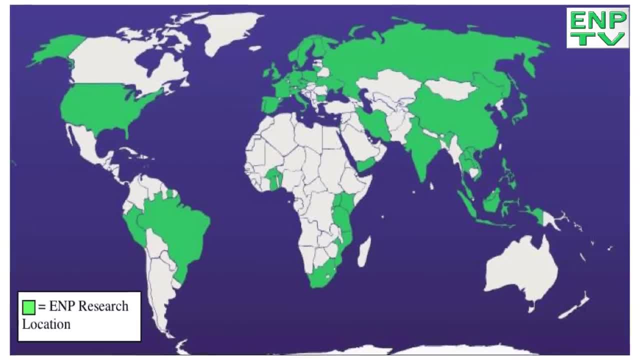 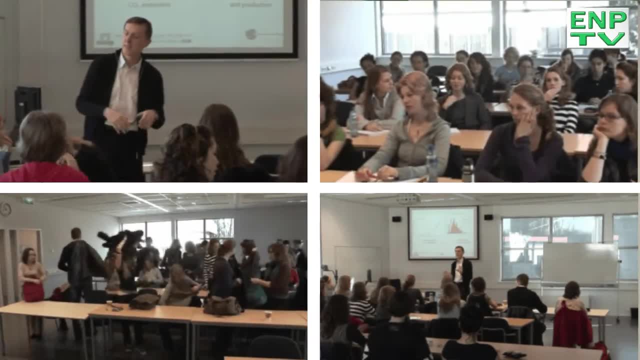 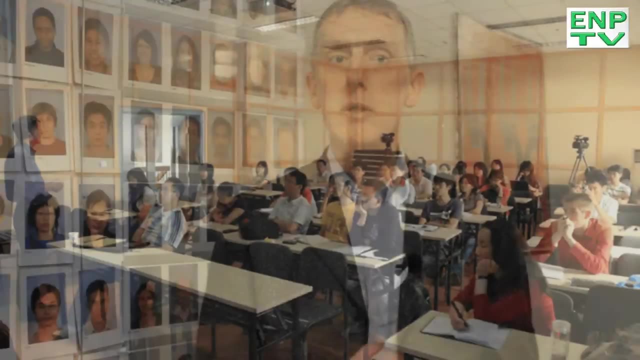 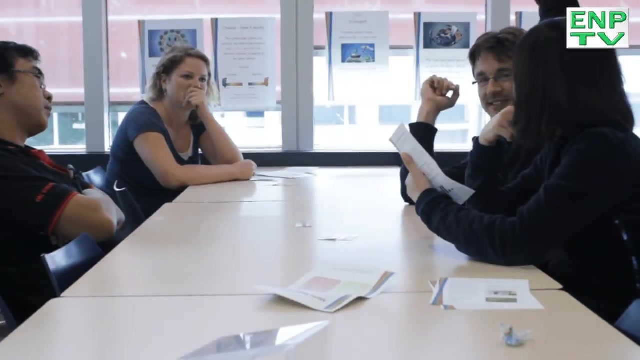 in Asia, in Africa, South America, Russia, the Pacific and Europe. Our international visiting scholars program, international student exchanges and the global international environmental lecture series bring staff and students from US, Asian, African and Latin American universities to our group. The 35 international master's students we attract every year often seize the opportunity to go overseas. 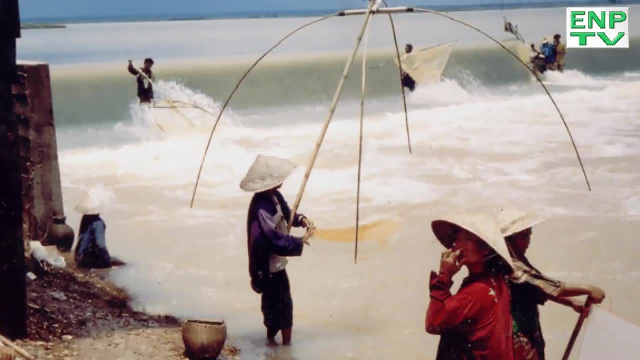 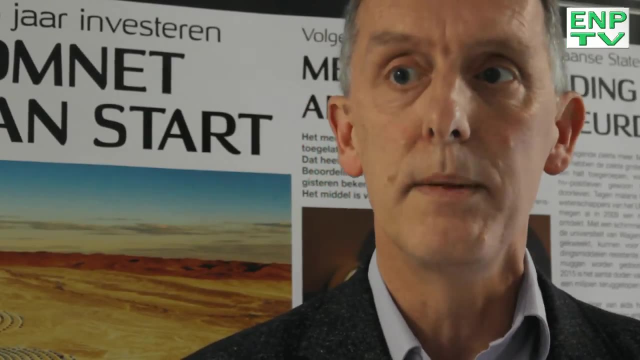 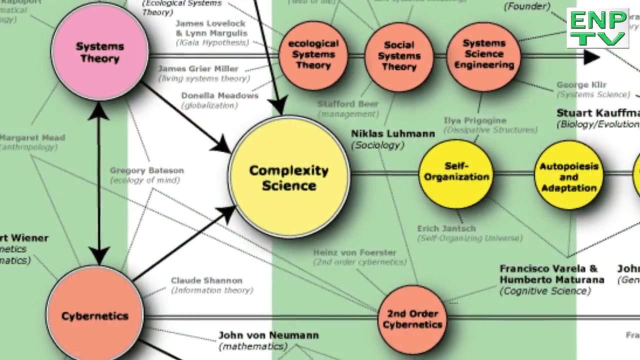 and work on challenging themes of the sustainable world of tomorrow. The staff at EMP has a diverse background in sociology, political science, environmental studies and human geography. We draw on various disciplinary approaches to lecture, understand and help solve environmental challenges, But we also work cross-disciplinary with economists, environmental scientists, ecologists and technologists. 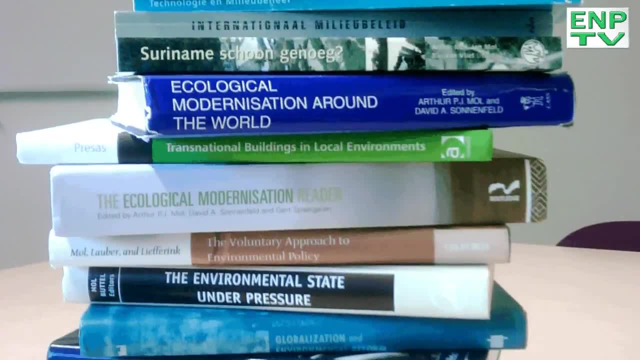 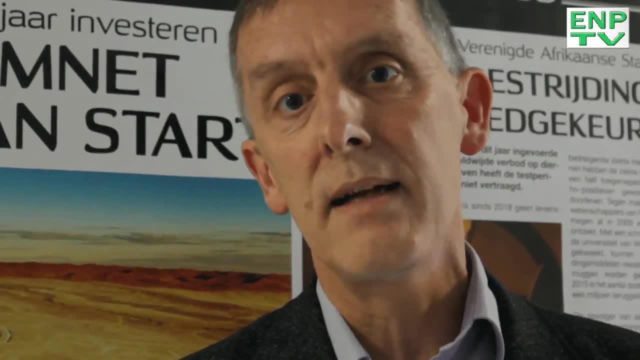 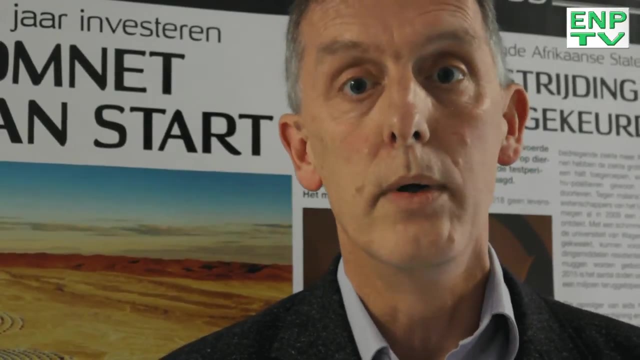 In a steady flow of high-quality peer-reviewed journal articles and books. we report on research, But we also provide advice to government authorities, international environmental NGOs and front-running companies on designing better governance arrangements and institutions for tomorrow. The research profile of the Environmental Policy Group can be grouped into three main areas. 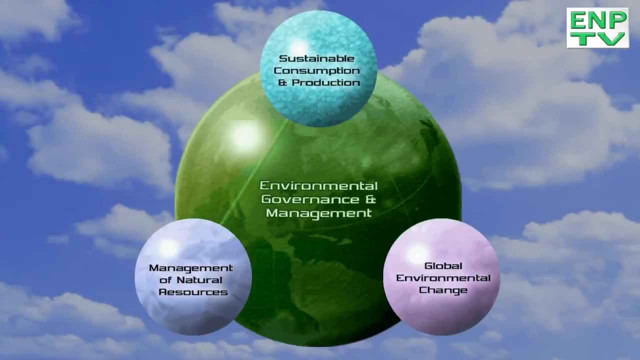 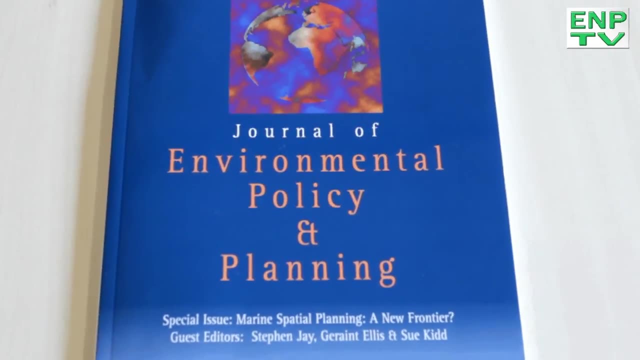 Sustainable natural resource use, global environmental change and sustainable production and consumption. Underlying these areas is a core interest in environmental governance and in social theory of the environment. Through our publications, we've been able to influence key theoretical debates in both of these fields. 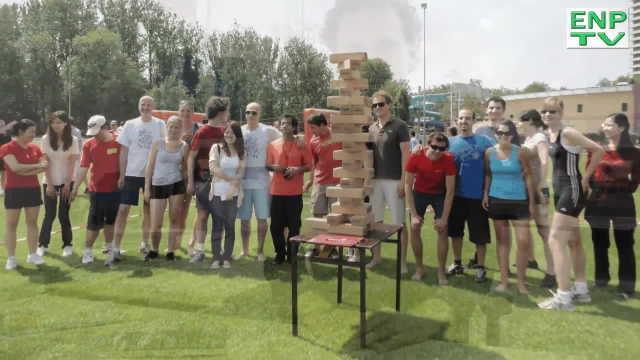 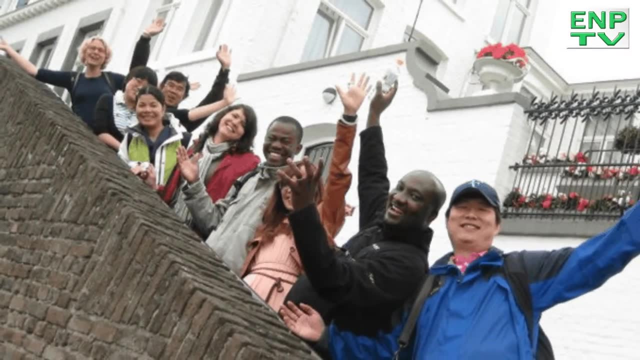 A key strength of the group are our PhD students, who come from all over the world and carry out fieldwork in a variety of terrestrial and marine settings. The diversity of PhD research and the projects our staff are involved in have allowed us to maintain high-quality research output. 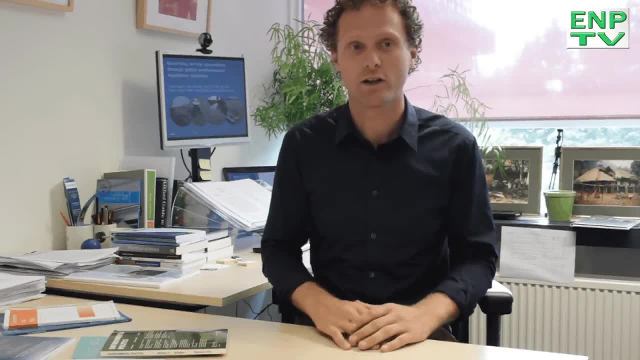 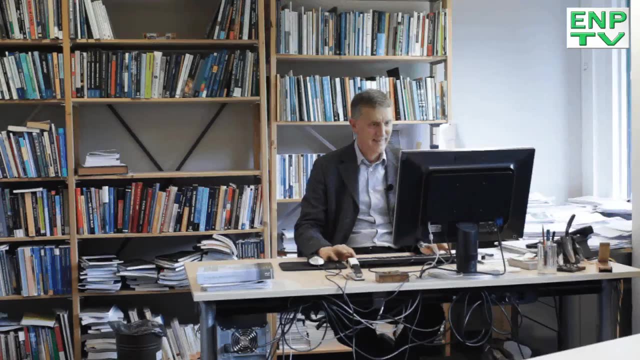 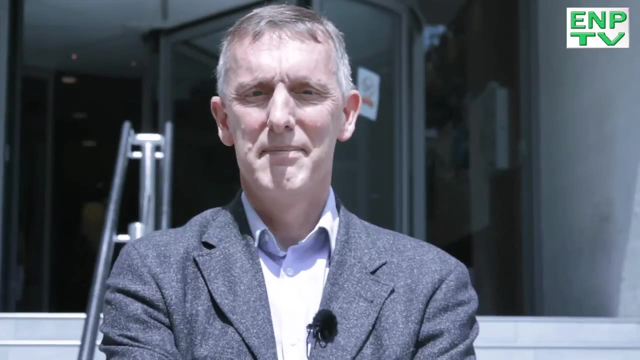 In the last five years we've been a top research group within Marketing University, and the Royal Academy of Sciences has also recognised our international contribution to the field of environmental governance. Our professor, Arthur Monk, has been recognised by both the International Sociology Association and the American Sociology Association for his contribution to the field of environmental sociology. 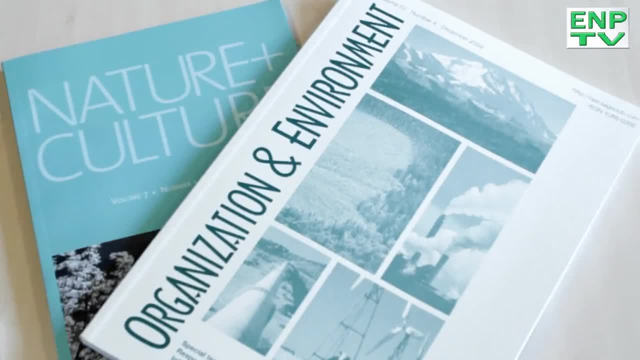 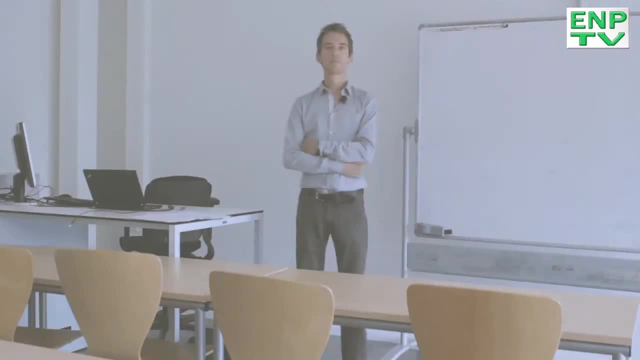 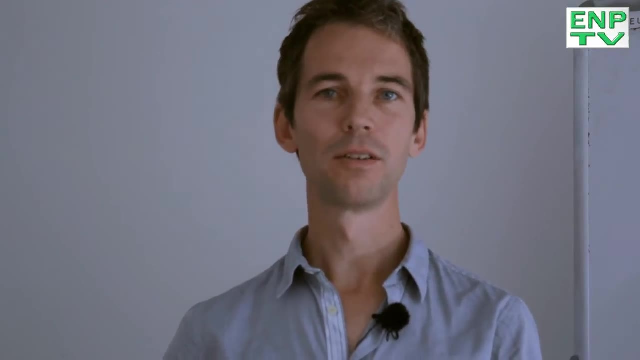 EMP staff are very active in the editorial boards of international journals, including Global Environmental Politics, Environmental Politics and Marine Studies. Hi, I very much like the wide character and variety of courses we do in the Environmental Policy Group, From individual thesis, supervision, tutorial groups. 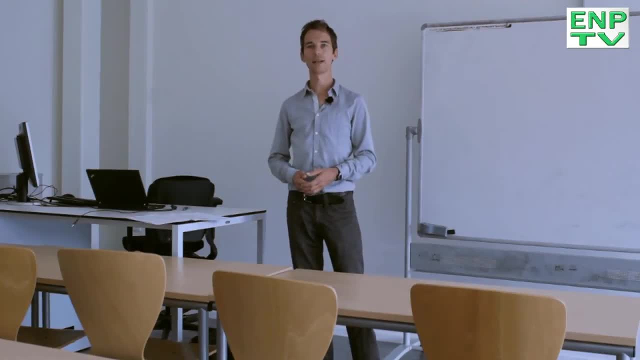 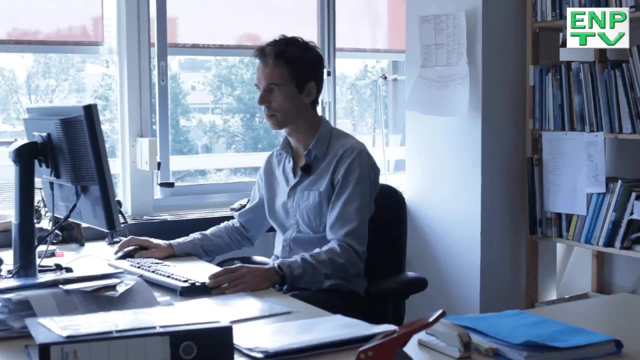 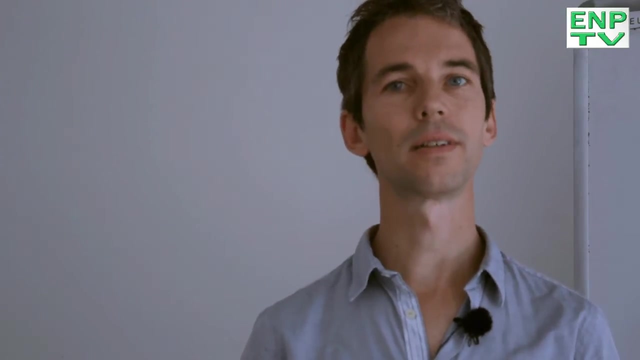 to academic consultancy, training and large classroom lectures. The Environmental Policy Group's educational profile is very wide, and our courses appear in five Bachelor's and ten Master's programmes in Wageningen University, including the Social Sciences and the Life Sciences programmes such as International Development Studies. 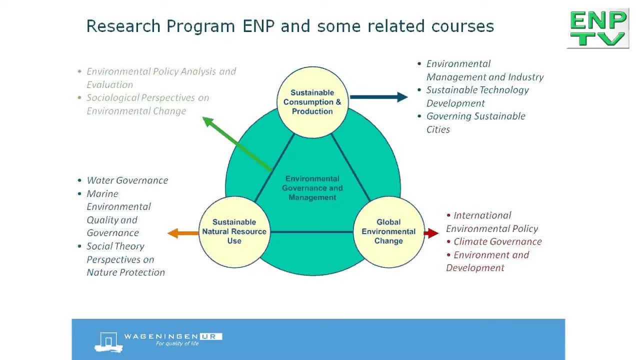 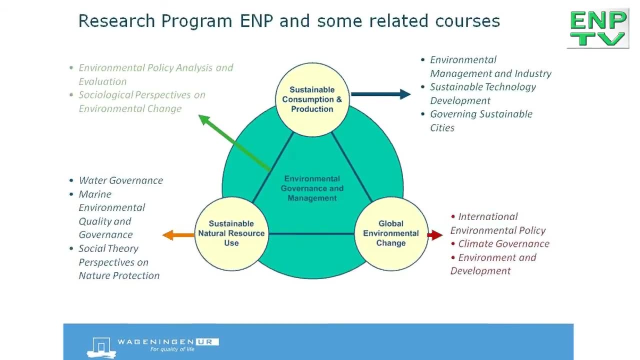 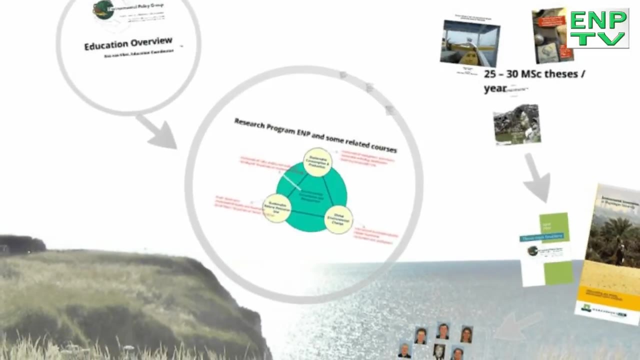 Climate Studies, Environmental Sciences and Marine Resource Management. Our disciplinary focus in all these courses is in sociology and political sciences, while many courses are interdisciplinary and taught together with staff from other groups in Wageningen, for instance, Rural Sociology or Environmental Technology. Students rank Wageningen as a top university for education in the Netherlands. 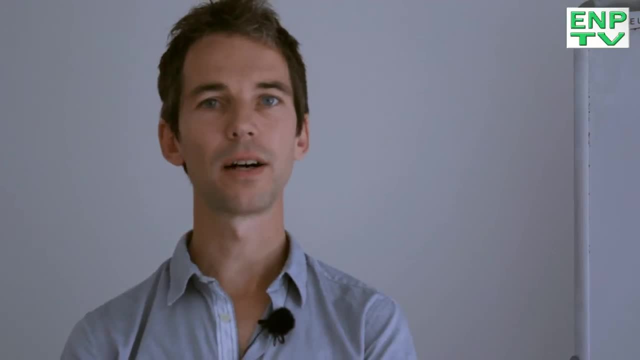 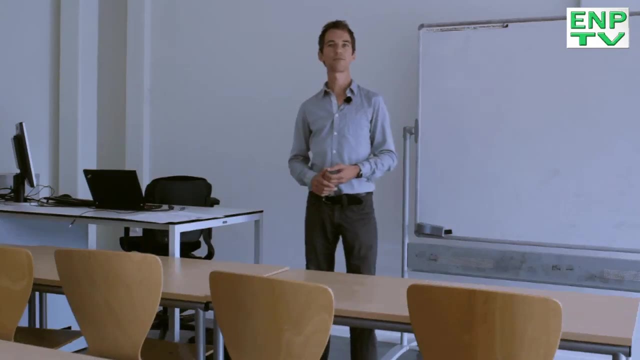 One key explanation for that is that we have a very high staff-student ratio and we maintain short lines of communication with students. As a lecturer, I find it very rewarding to work with such a variety of students from all over the world, with so many backgrounds. 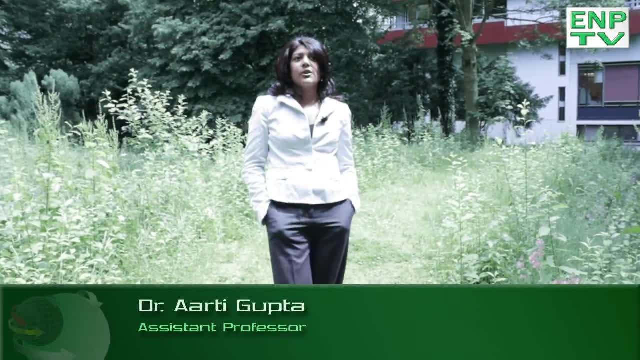 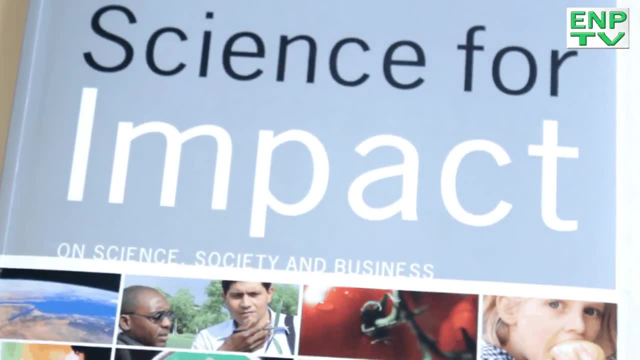 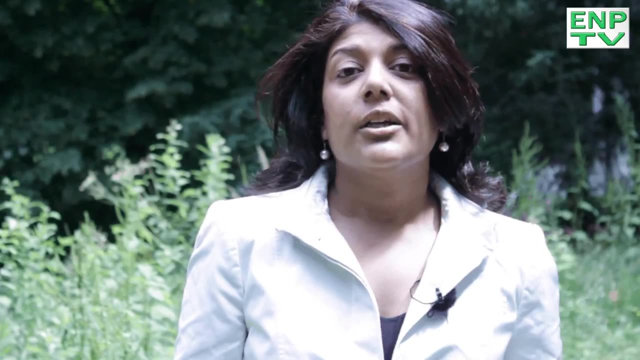 At ENP, we also care about the social relevance of our research, what we call here science for impact. For example, in two of our large research projects, Provide on urban waste infrastructures in Africa and Best Tuna on sustainable tuna- ENP researchers work directly with decision makers in both sectors. 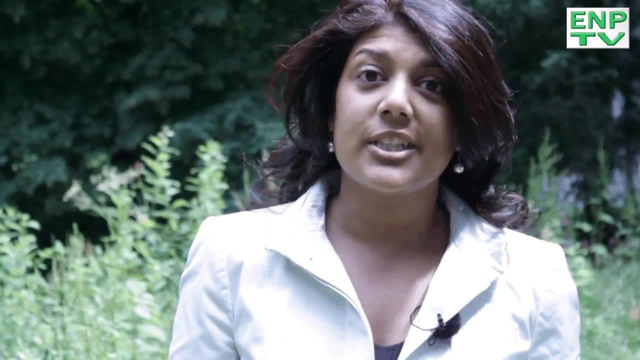 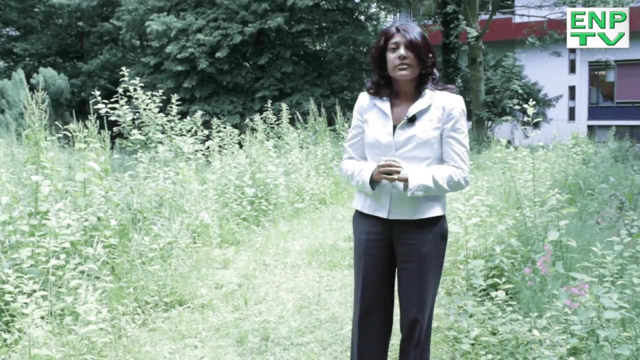 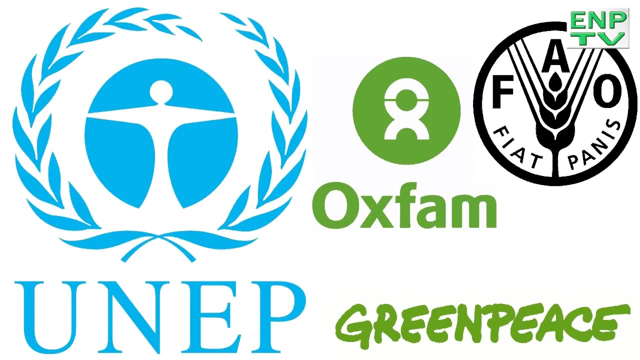 to make sure that our research is also relevant in real time. Of course, we also have impact through our graduates. Our MSc and PhD students are spread across the globe working for consultancy companies, government ministries, international organizations and NGOs. This far-flung global network ensures the continual application.